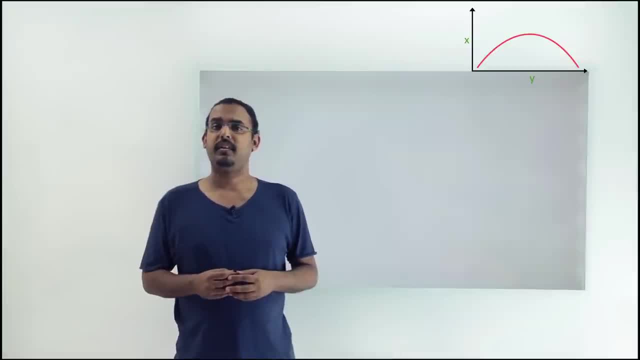 Have you seen this shape elsewhere? Are you familiar with this shape at all? I bet a lot of you like playing or watching cricket. Does this shape not resemble the shape of the path of a ball when a batsman hits the ball for 6 runs? 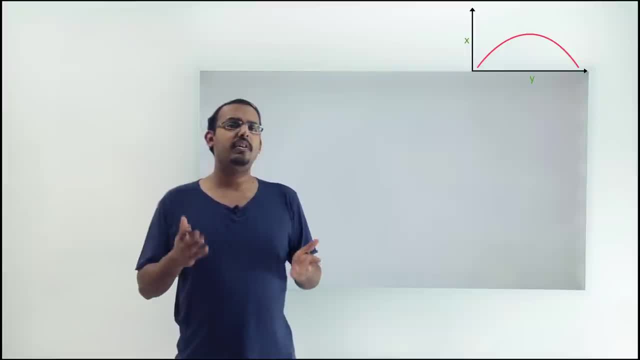 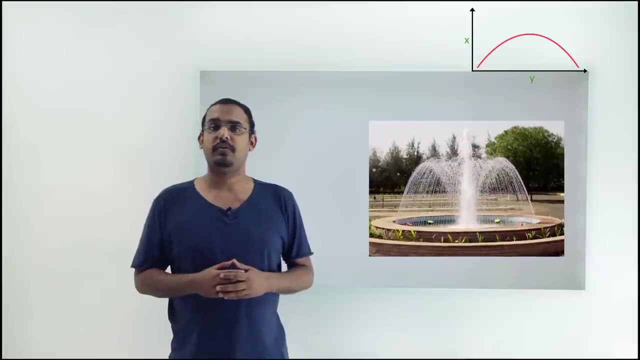 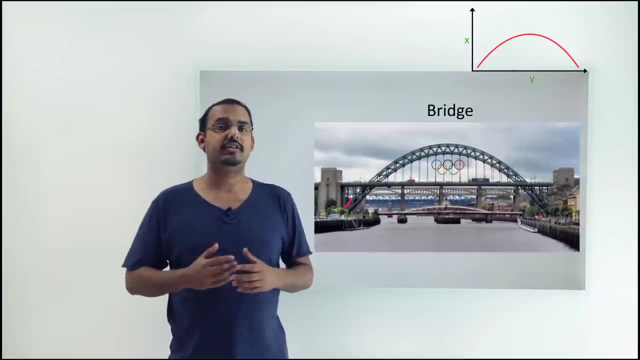 It does resemble that shape right. If you observe closely, you can find the presence of this particular shape all around us: The shape of the path of water when it comes out of a water fountain. The shape of the structure of many bridges all across the globe. 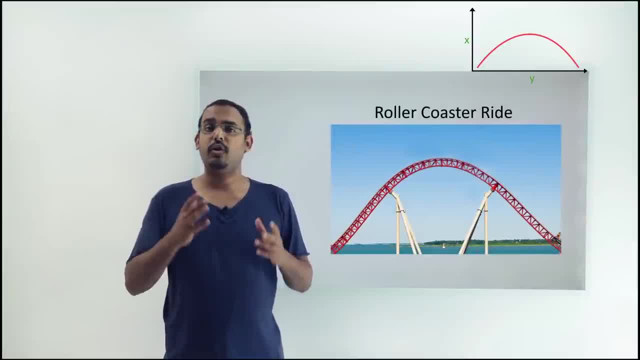 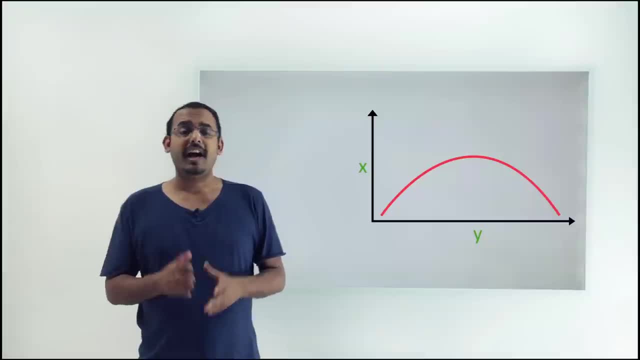 The shape of the roller coaster rides that we all love to ride in amusement parks. They all resemble this particular shape, right? But you might be thinking: why are we talking about this particular shape while studying Quadratic Equations, If you recall correctly, in the chapter of Polynomials? 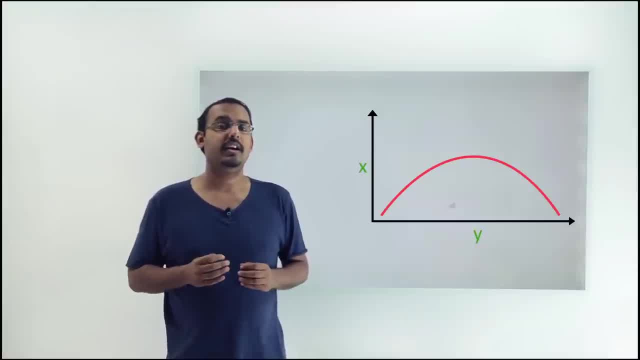 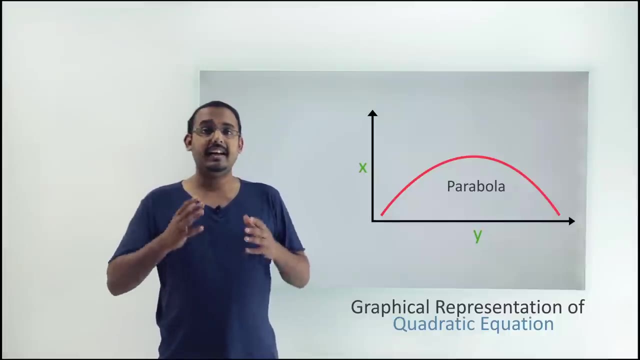 we have seen that this particular shape is what we call a parabola, And a parabola is used to represent a quadratic equation in graphical form. As you have already seen that there is a vast and diverse scenario of real-world applications related with the shape of parabola, 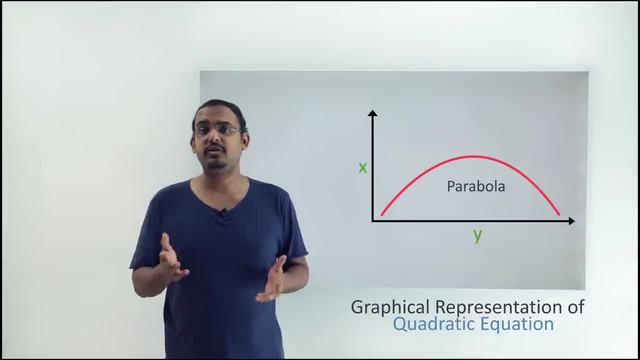 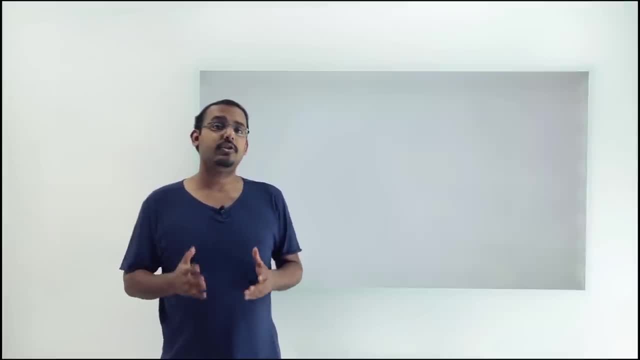 the study of Quadratic Equations for analysis of those shapes naturally becomes very important. To begin our journey into Quadratic Equations, we'll first look at what Quadratic Equation actually is. Then we'll go on to some basic terms of Quadratic Equations. 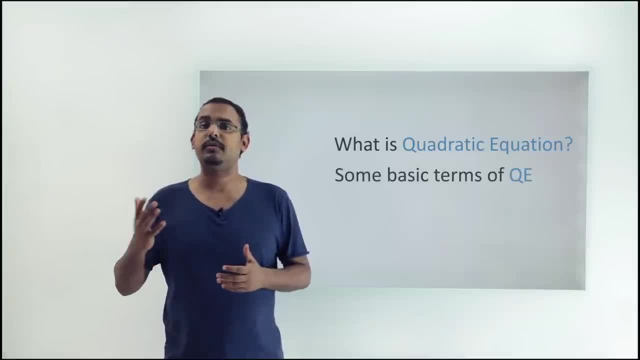 We'll see what we mean by saying solving of a Quadratic Equation. We'll see what the roots of a Quadratic Equation are. Then we'll go on to study about the three different methods we have for solving Quadratic Equations. After that we'll have a look at the different kinds of natures of the roots of a Quadratic Equation. 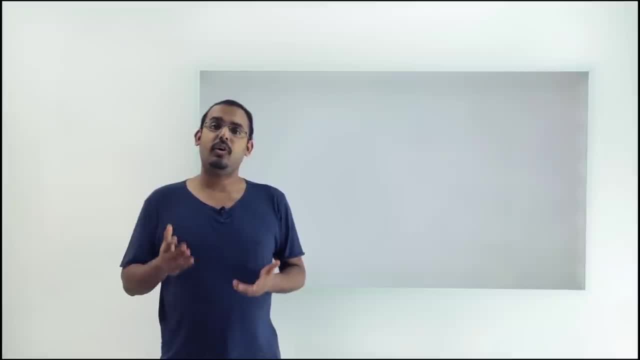 Once we are through with all the concepts in the chapter, we'll do some solved examples To understand the concepts of Quadratic Equations better and to apply them in real-world scenarios. See you in the next lecture.